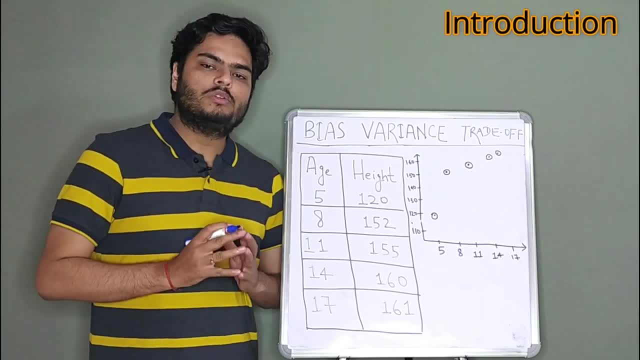 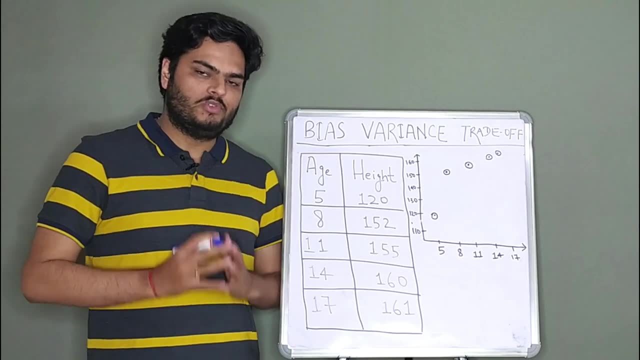 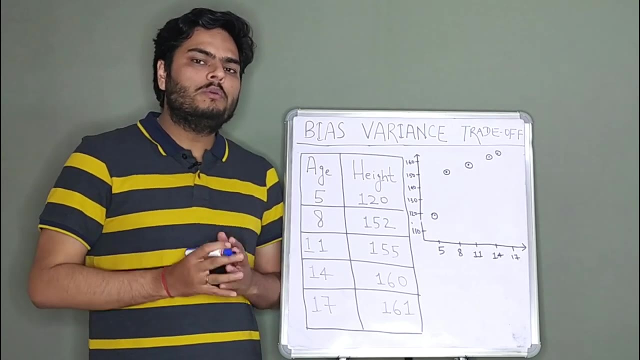 Bias variance trade-off- One of the must-know concepts for every data scientist and one of the famous interview questions for almost all data science interviewers. So what is bias? What is variance? What is the meaning of bias variance trade-off If we know how a machine learning model 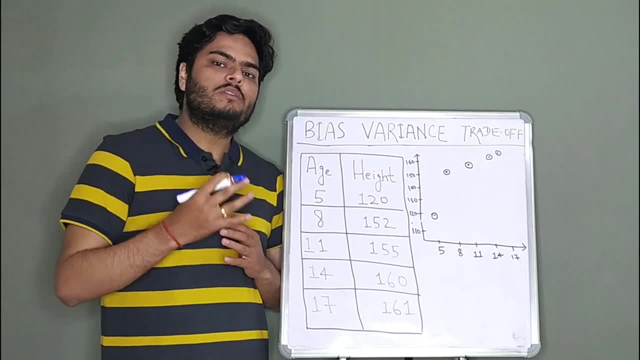 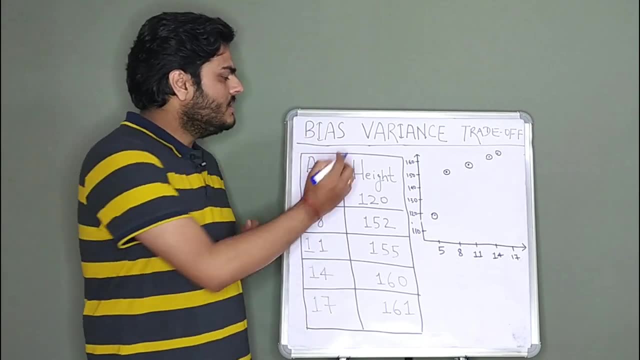 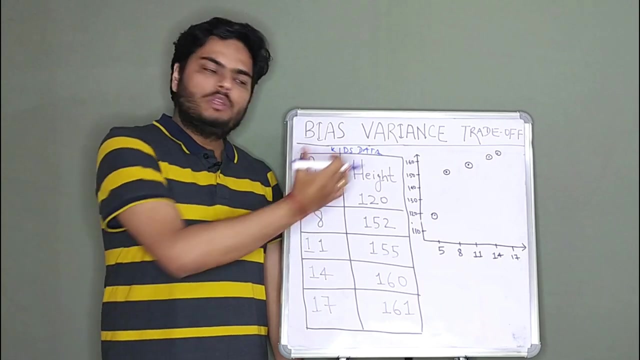 works, then can I tell if this model will have high bias or high variance? We will know answer to all these questions with a simple data. So what you can see here is a kid's data. So this is kid's data, where on x-axis I have the age of the kid, on the y-axis I have the height of the. 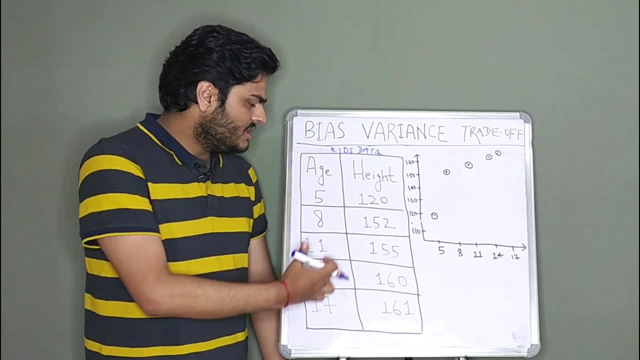 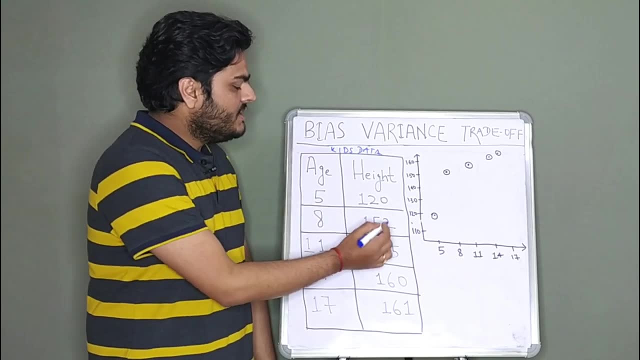 kid. So all of us know that beyond a certain age, height of the kids will not increase that marginally. So, as you can see, from 5 to 8, the height is going from 120 to 152.. On the other hand, if you see from 8 to 11, the shift is low. 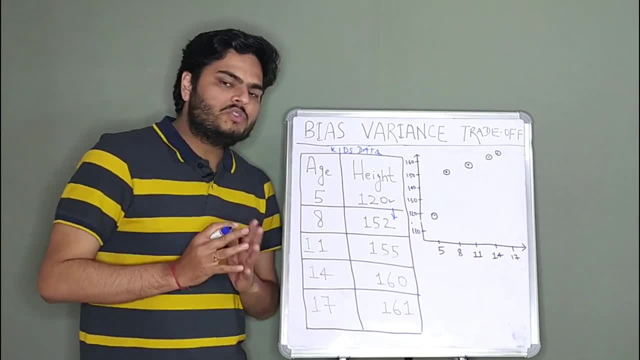 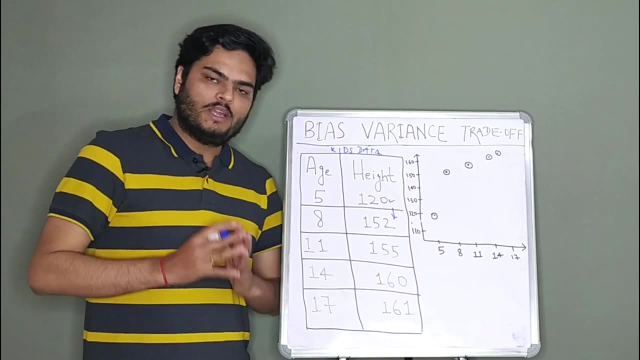 So I have knowingly created a data like this and we will understand everything about bias and variance using this simple data. Welcome to Unfold Data Science. My name is Aman and I am a data scientist. Let's start the discussion. So I have plotted here, If you can see on the y-axis. 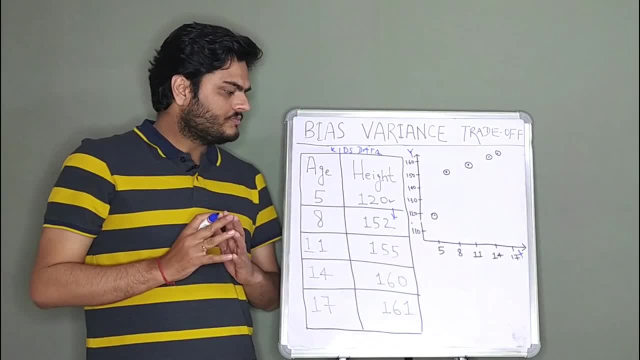 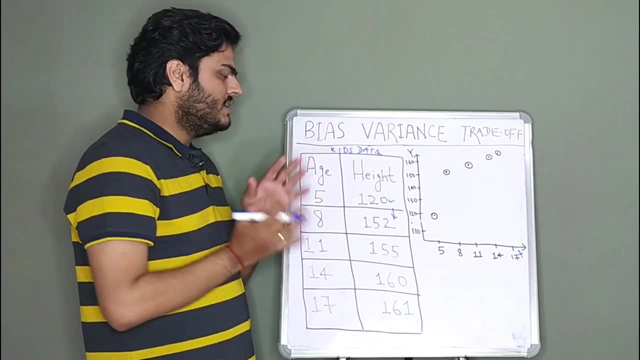 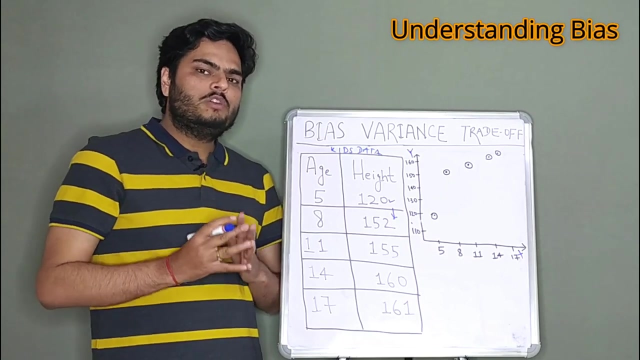 I have height. On the x-axis, I have age. Okay, Now let us say, I tell you, fit a model, any model of your choice, fit a model on this data. you know to predict the height, weight of the person given the weight of the person. Okay, So what you will do, let us take. 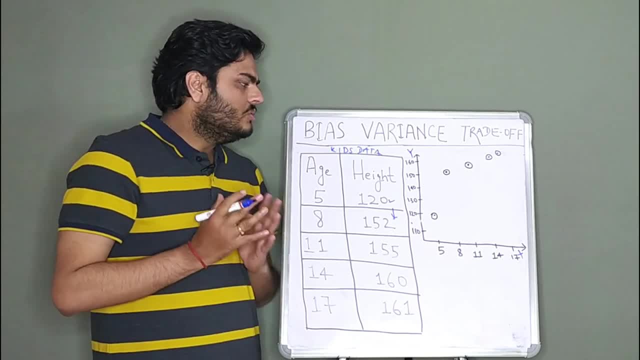 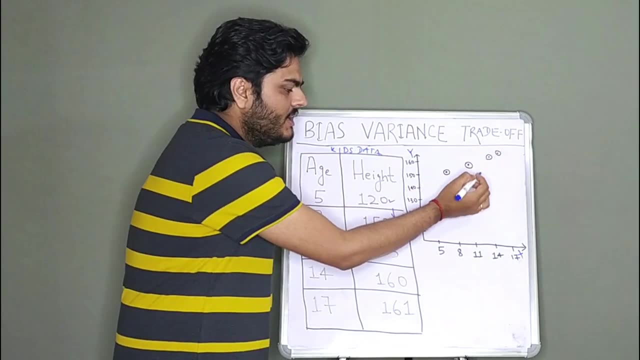 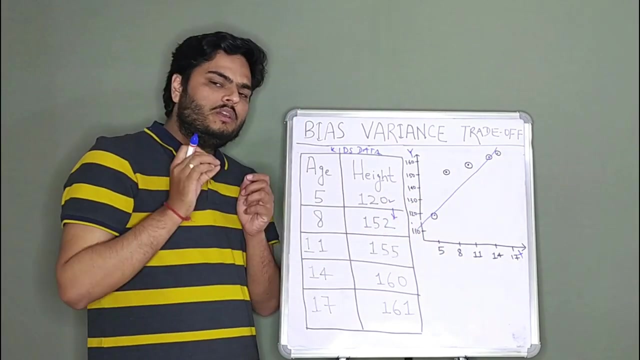 the example of very simple linear regression model. Okay, So a linear regression model is nothing but a line. Okay, So let us say these are the data points. We take a line and let us say this is our linear regression line. Okay, This is our linear regression line. Now linear regression. 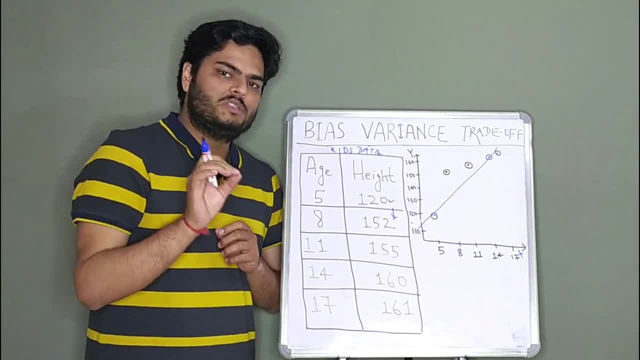 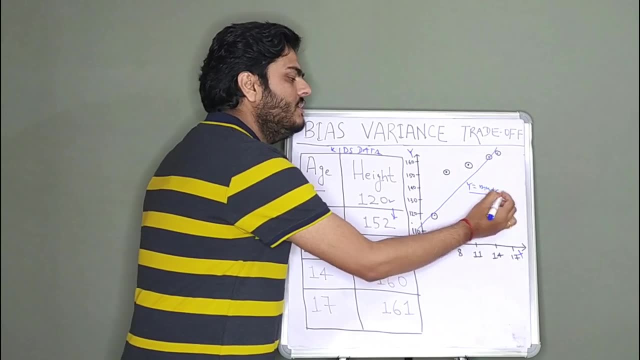 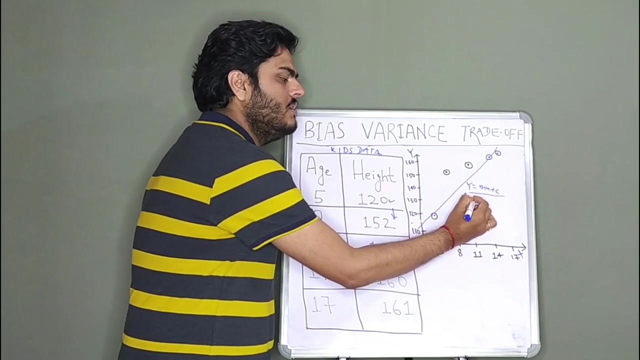 line is nothing but an equation of the form: mx plus c. Right, This is a line. So this line is: y is equal to mx plus c, Right, This is, in the simplest form, equation of a line. Now, this is nothing but a function of x. You can also say: fx is equal to mx plus c. So when the model fitting 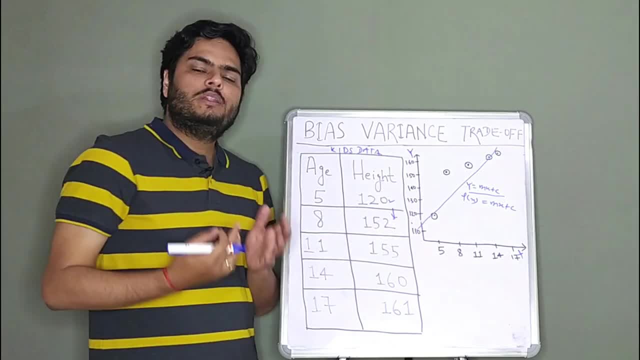 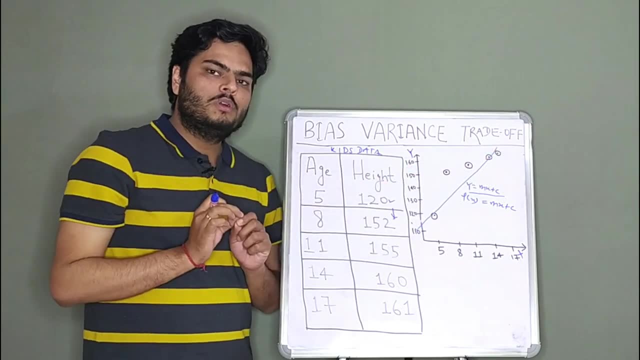 happens. we get to know what is m and what is c, And then, by any given x, we can compute y or fx. Right, So this is my fx, this line. Now why I am explaining you. this is the moment we say: 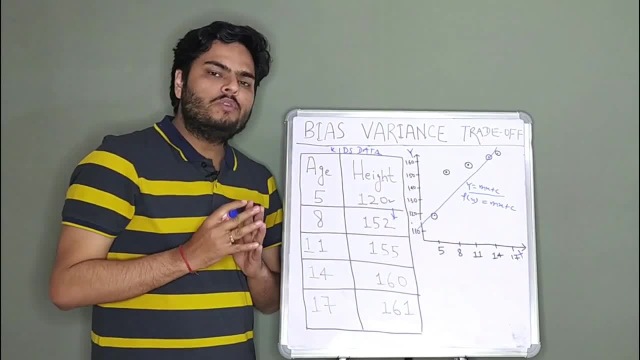 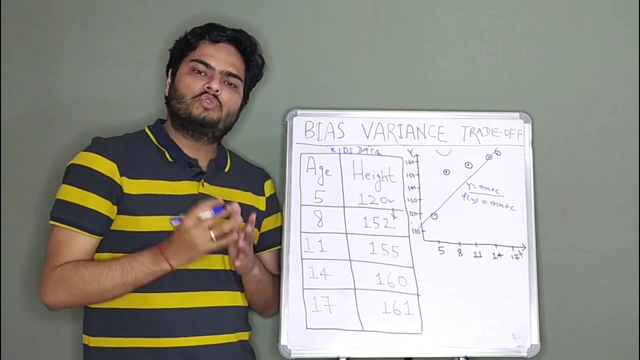 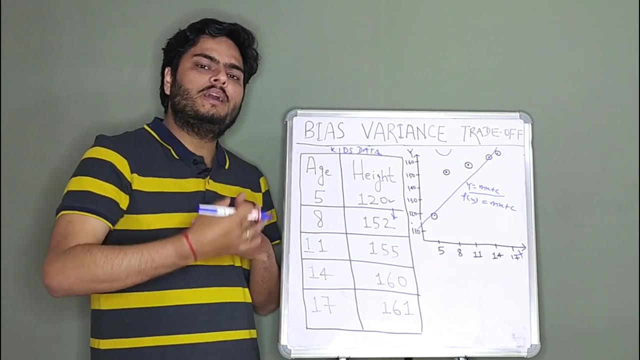 fx. the moment we say a function, a function will have a form. Right, So this is a linear form. This can be a parabola form, Right, Something can be a squared function, Something can be a cube function, So function has a form. So when do we say a model is having high biases? 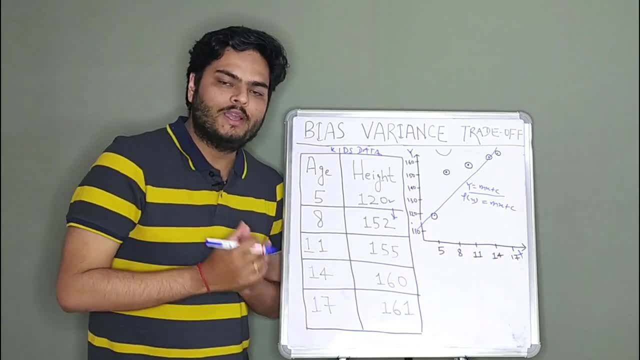 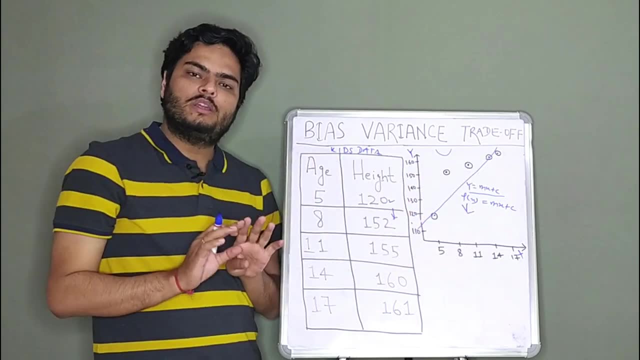 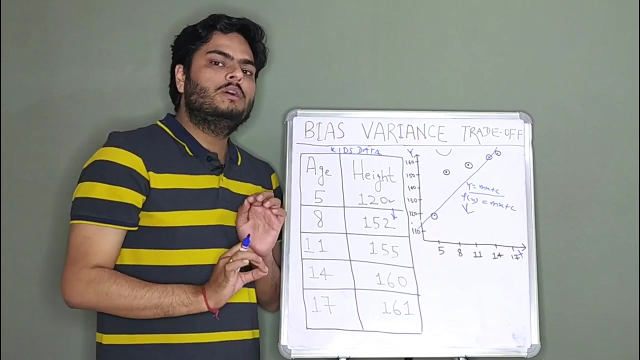 When the form of the function is biased. I will repeat it again: fx is the function which is fitting on this data. when you fit a linear regression model, If there is an underlying assumption about the form of the function, then we call that model is a high bias model, which means model is biased towards that form. 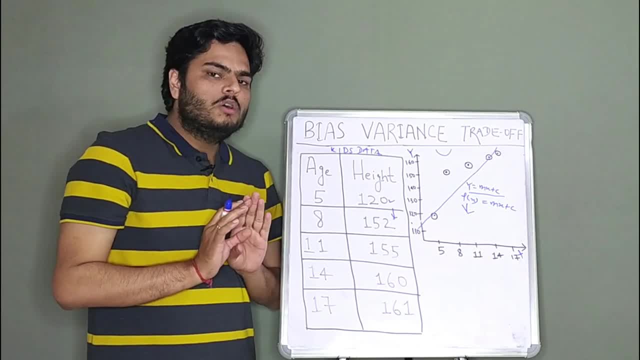 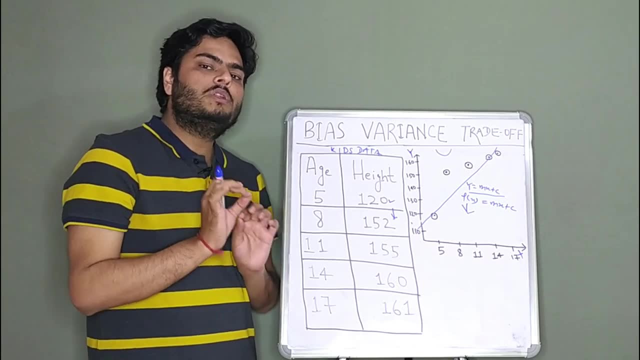 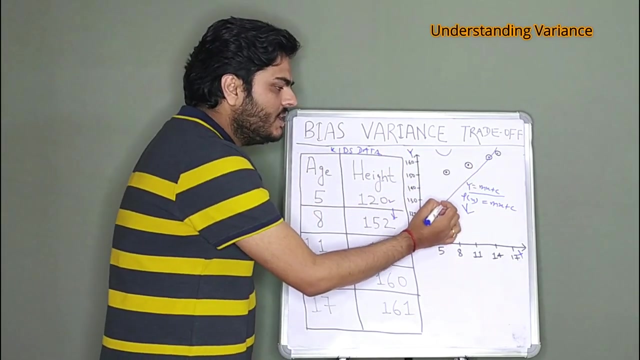 What is that form? here? The form is the linear form. Okay, So this model is said to be high bias model. The reason for that is there is a underlying assumption about the form of the function. Now, what is the other way? we can fit a model on the same data. Let us say you take 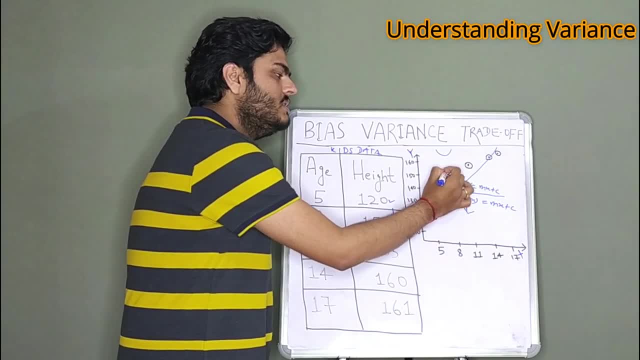 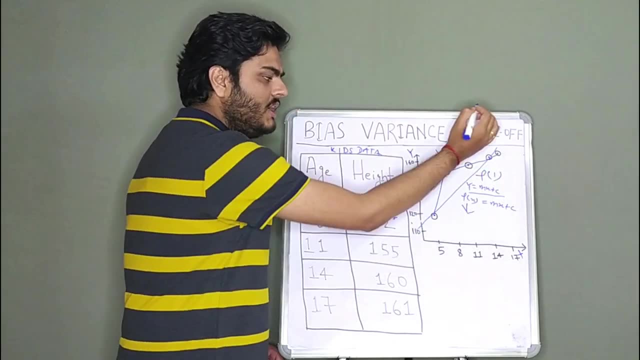 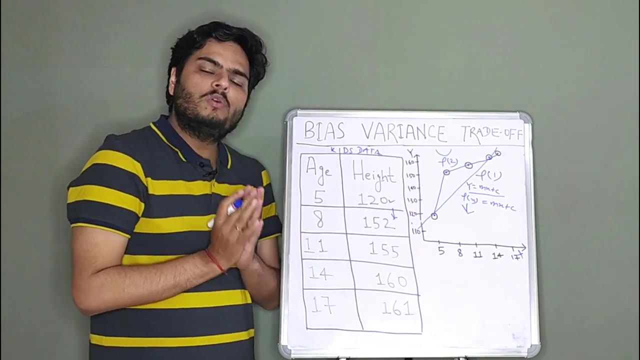 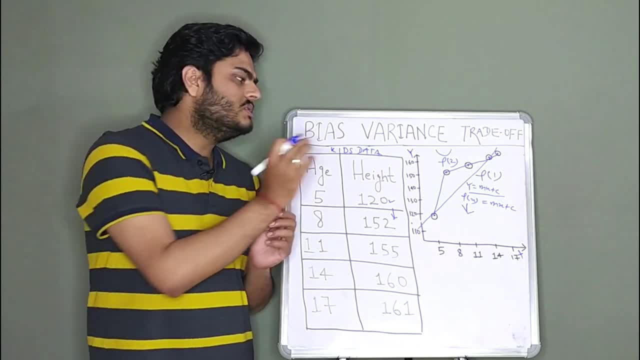 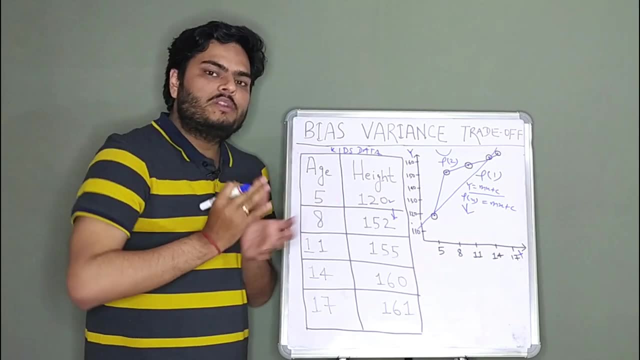 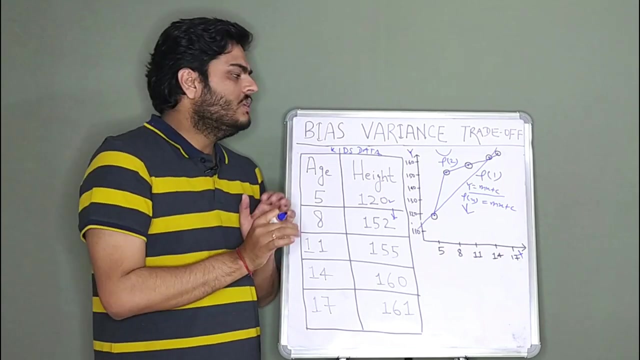 necessarily linear. it is not assuming any form, it is just going as the training data is going. so whenever your function is too much following the training, then your function or model is said to be a high variance model. now, what is the difference here, guys? so if you see this, f1 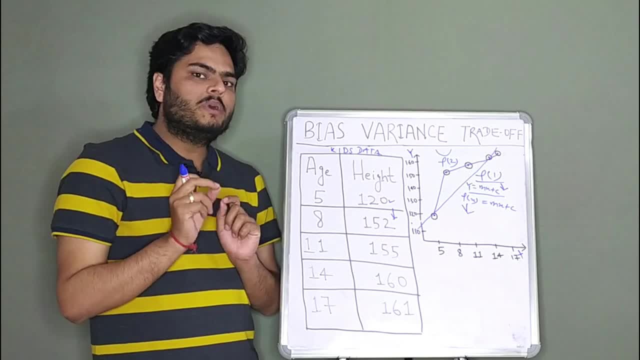 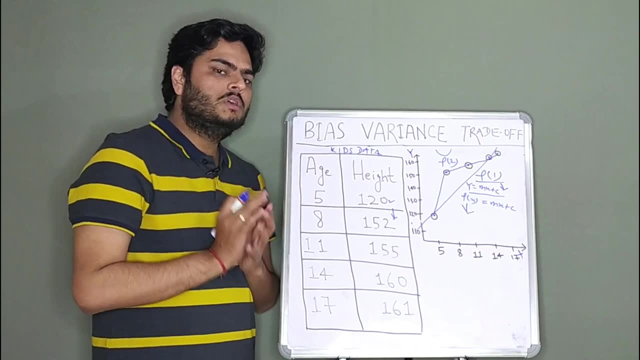 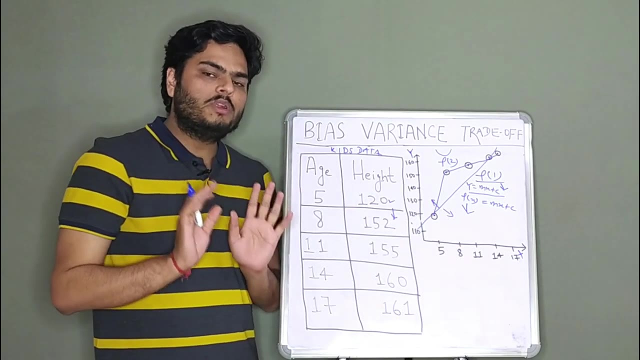 is a generalized function, so high bias model will be a generalized model, which means tomorrow, if new data comes, new training data comes, then what will maximum happen is this line will shift little bit toward this side or little bit towards up. this is about high bias model. what happens to the high variance model? let us say 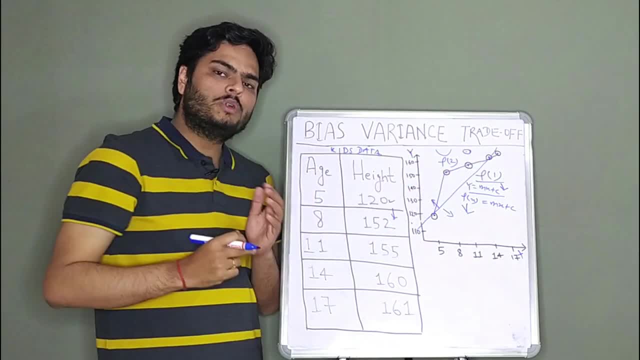 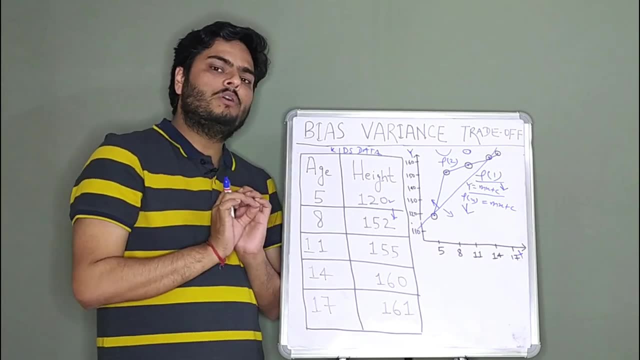 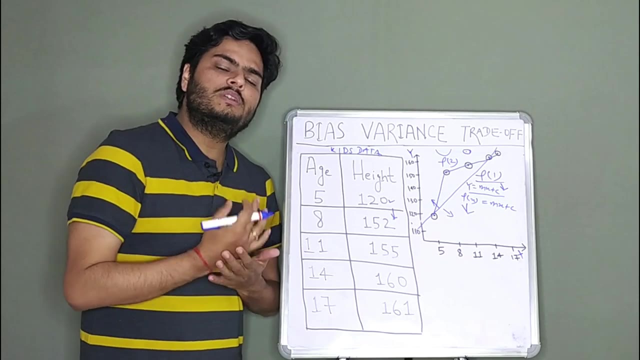 a new data comes. new data comes here. what will happen is your entire function will change. that is the issue with high variance models. let us take example of some of the high bias and high variance model. so, to keep it very simple, if you have to recollect which function have high bias, 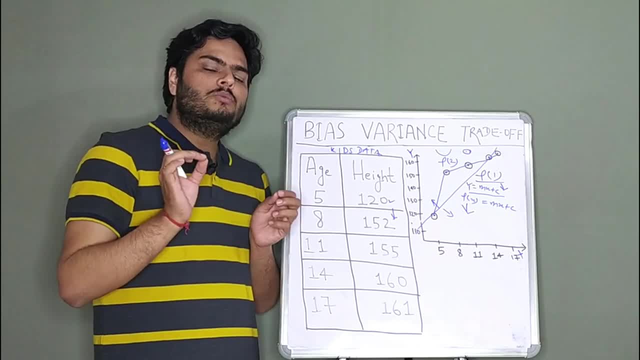 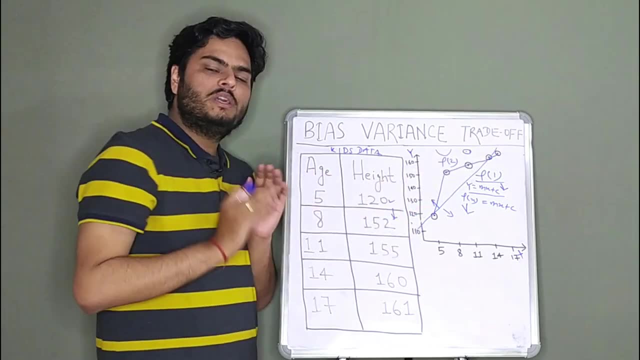 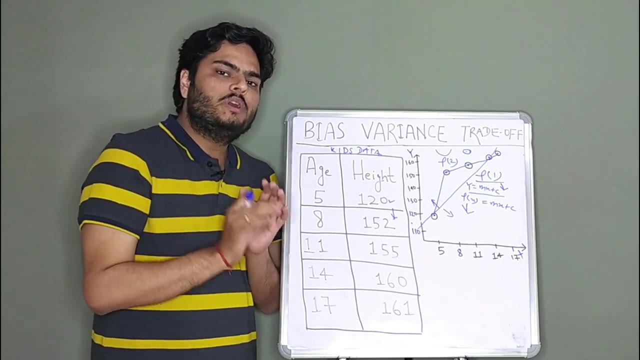 then you have to simply think which function assume: a form of the form of the data or a form of the method? right, linear regression assumes there is a linear relation between x and y. logistic regression assumes there is a linear relation between logit and mx plus c. right so? 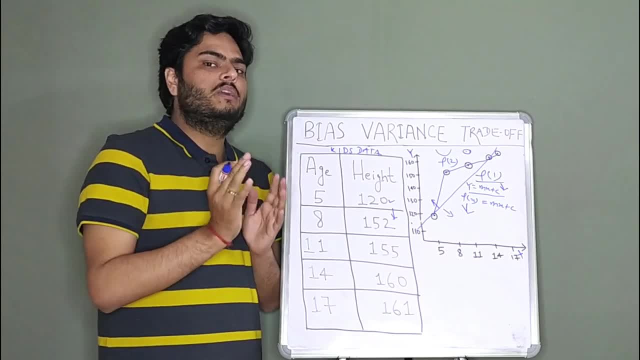 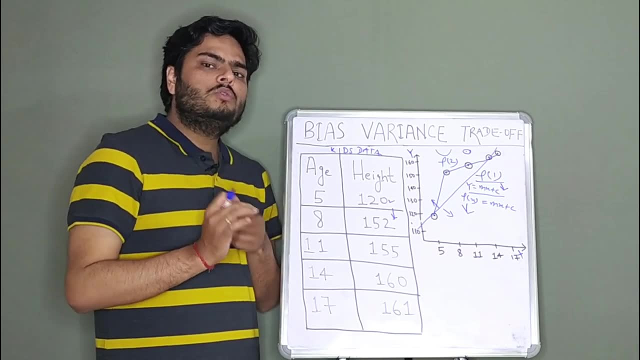 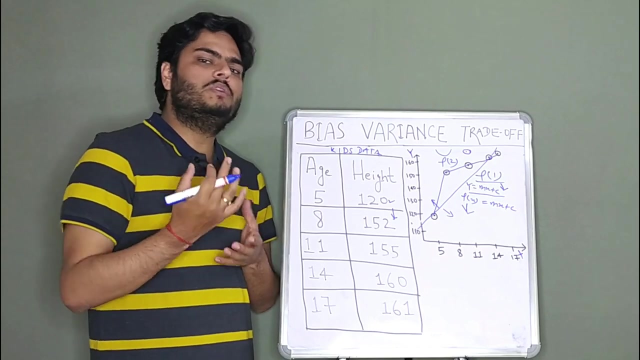 anywhere, you see there is a form that becomes a high bias model. what will be the example of high variance model? all those machine learning models where there is no form defined of the data, no, you form assumed of the data, for example, decision trees, for example your svm models, for example. 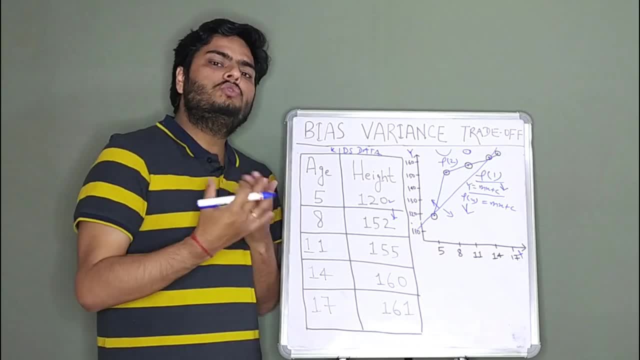 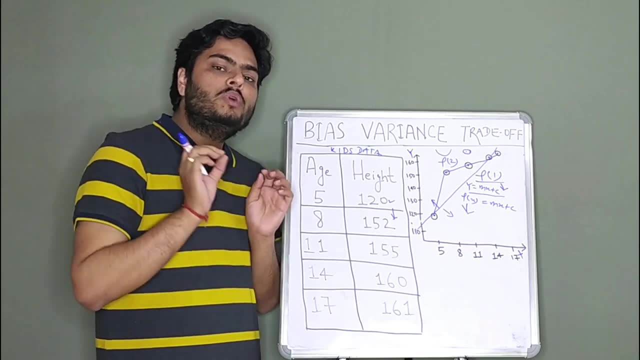 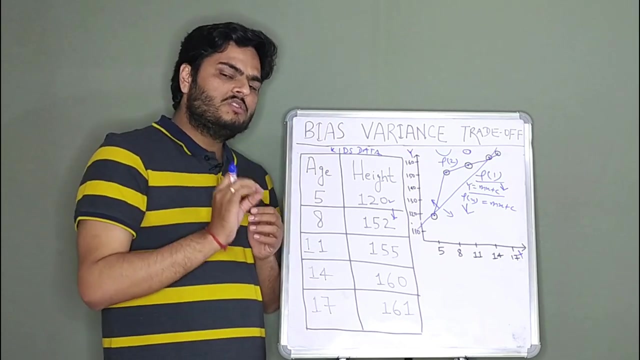 your k nearest neighbors. these models do not assume the form of the data or do not undergo and try to fit a line or a function to the data. with the assumption of the form, those models are called high variance or low bias. it is basically vice versa: high variance model will have low bias. 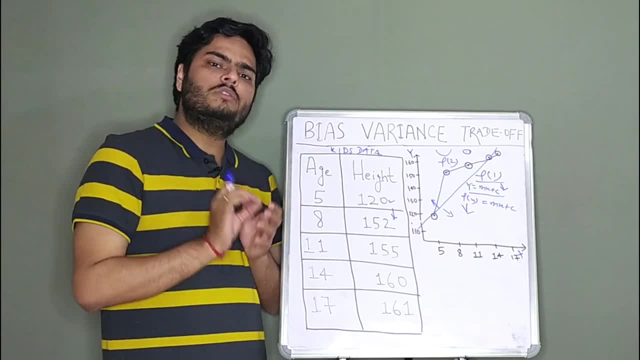 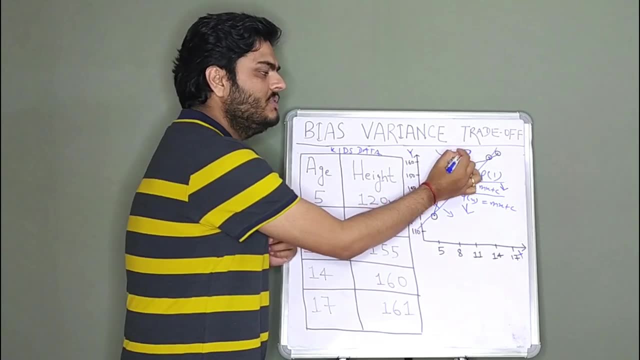 and high bias model will have low variance. what is the definition of variance? a model is said to have high variance. if, at the moment, i change the training data, like i give you the example, if a new point is added, then your entire model changes. so what is what is model? in this case, this line. 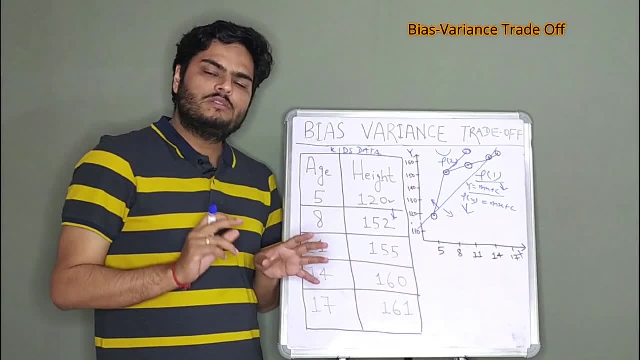 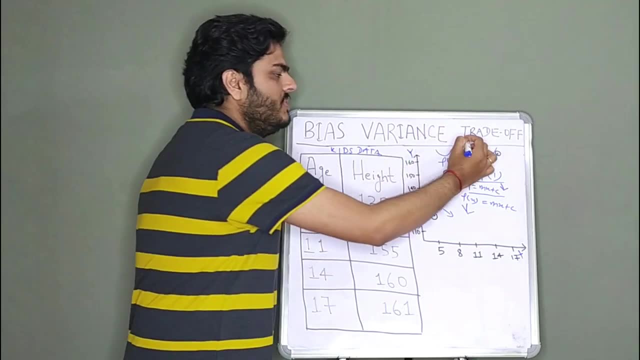 so f2 will have to pass through this, hence the entire f2 will change. now what is the meaning here to understand is what is bias variance trade-off? so, as i told you, models with low bias model will have low variance and high bias model will have low variance and high bias model. 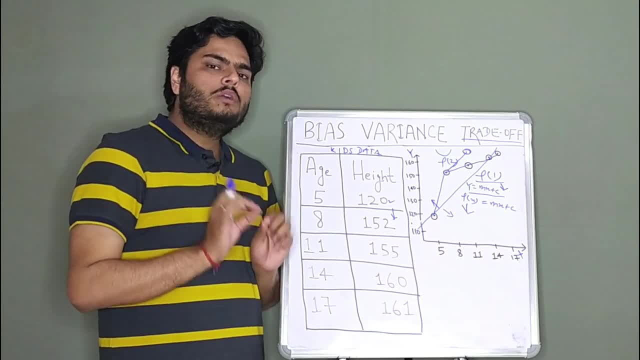 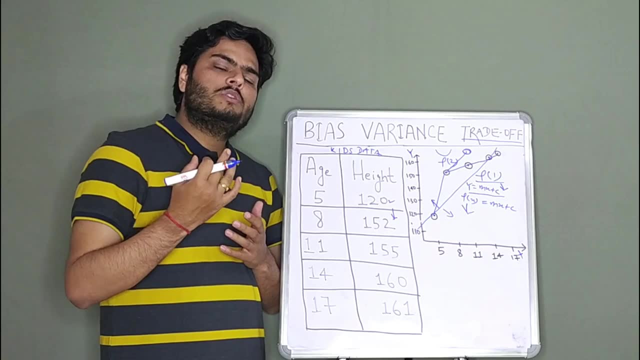 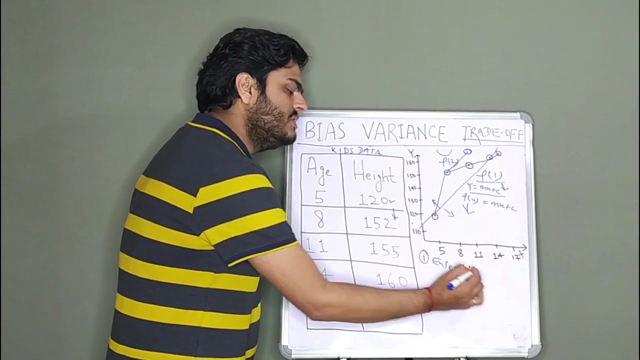 will have high variance. high bias will have low variance. what we should have ideally is low bias and low variance. how to achieve that? so you must be aware of some of the ensemble techniques, right? so ensemble techniques like bagging, boosting, stacking, those kind of techniques will help you in reducing 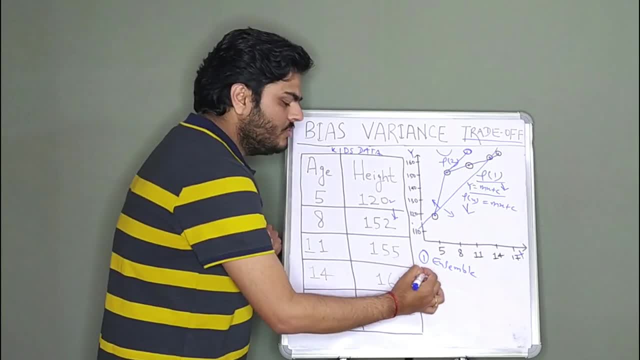 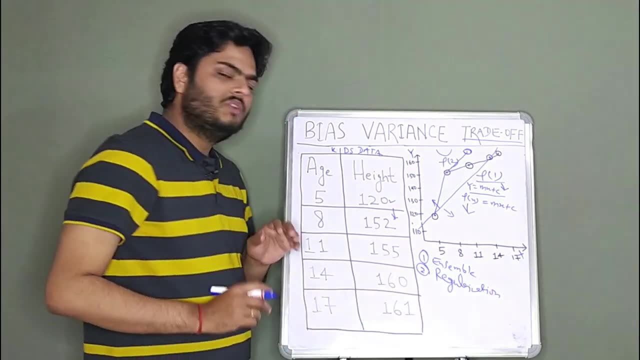 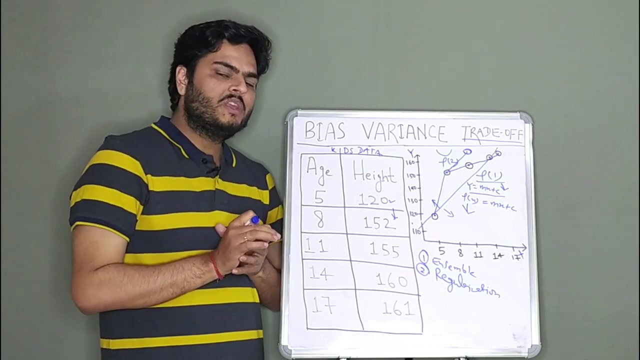 bias and reducing variance as well. next, what you can do is you can use regularization in regression right? so if you have heard of lesser regression, least regression, those regression will help you in achieving a lower bias and lower variance in your model. okay, few more things to keep in mind. 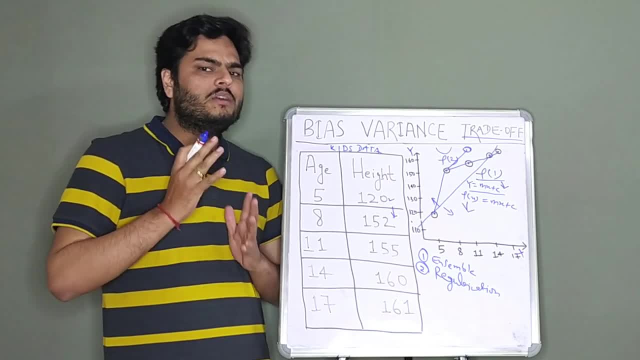 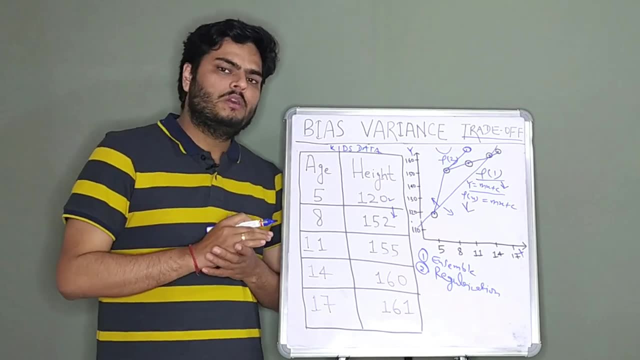 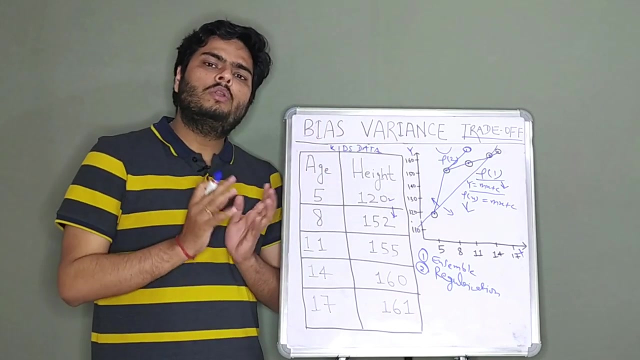 here is. high bias model will normally under fit your data under fitting means. it might not give you very good accuracy on your training data and test data as well. on the other hand, high variance model might give you a very good accuracy on train data, but not good accuracy on test data. 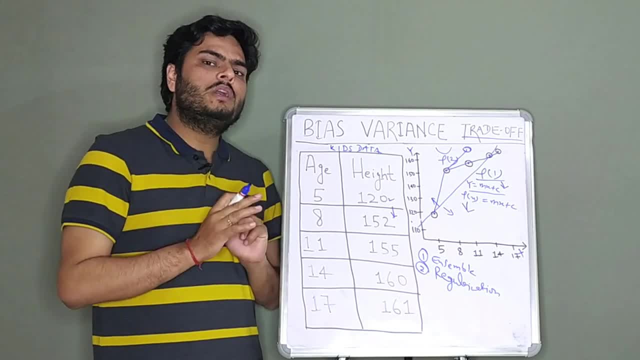 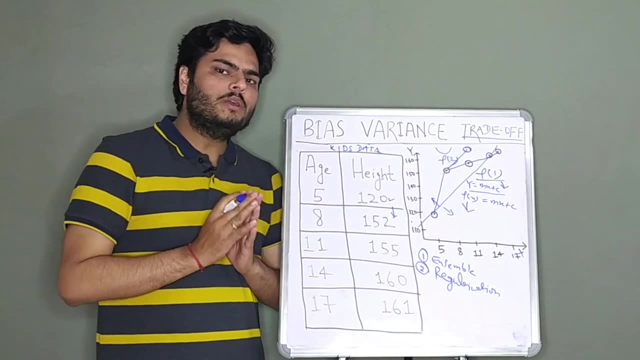 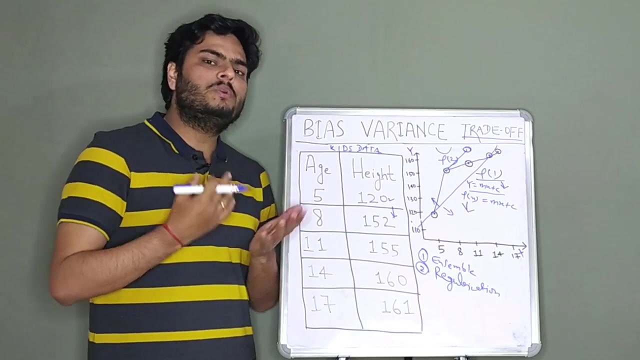 or when you expose this to new data. this phenomena is also called as model over fitting, when your model is doing good on train and not doing good on the any unseen data. okay, that is number one. number two is high bias. model will be simpler to understand, to manipulate, to work with. okay, so, as 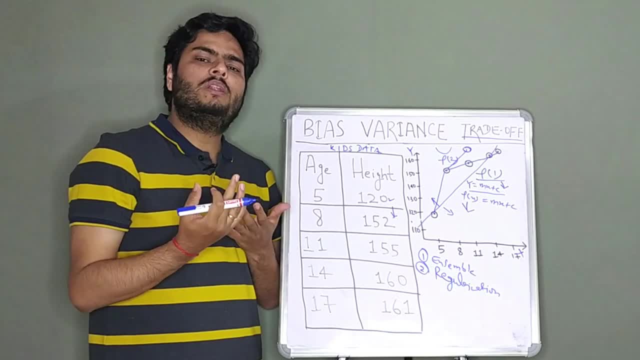 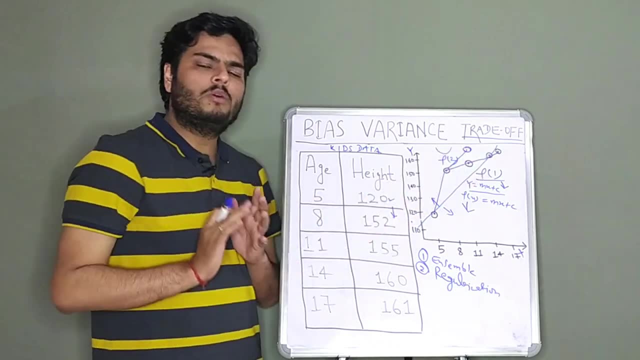 you can see, this is a line. this is having high bias. hence it is simple, it is not very complex. on the other hand, high variance model will be little complex. okay, as you can see, this is f2- little complex, right? high bias model will be more generic in nature. you can generalize it. okay. high. 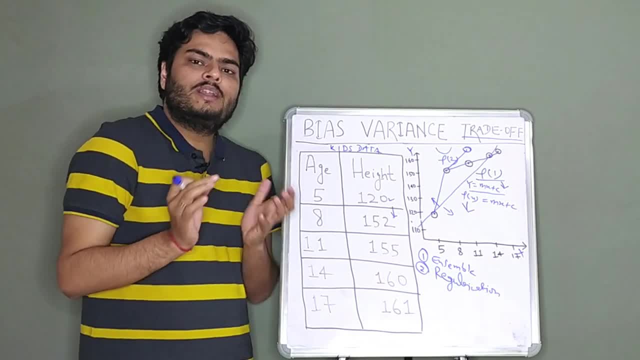 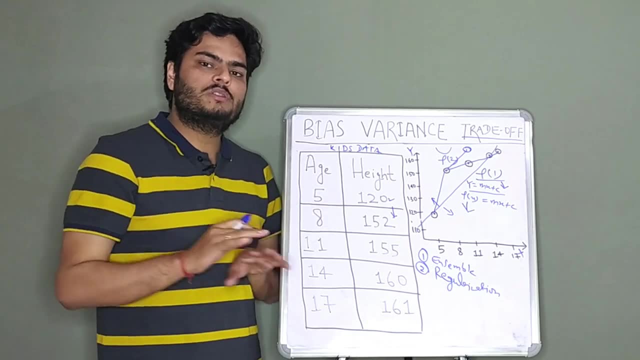 variance model will be less generic in nature. you cannot generalize it on multiple data sets. the last and the final point you should keep in mind is: if you forget all these concepts- let us say in interview this question comes to you suddenly- remember just one point: any model which 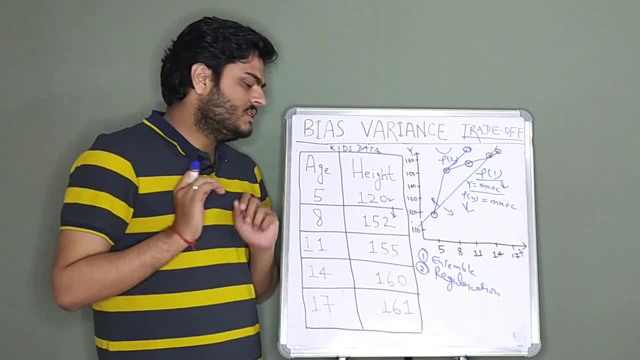 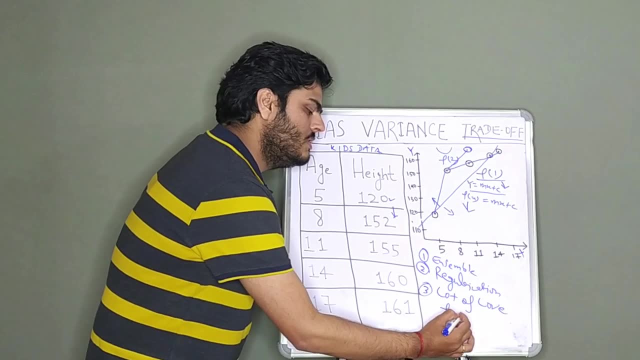 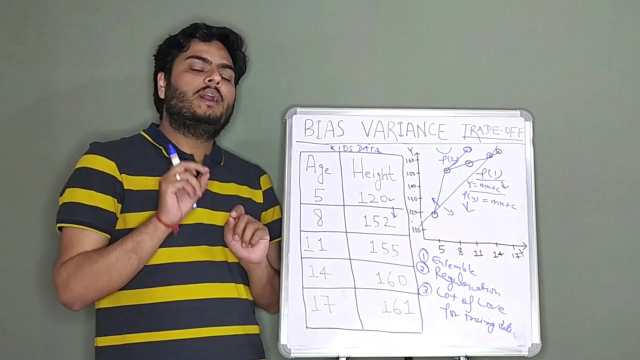 has a lot of love for the training data. okay, I will just write it down. just remember this one point, guys: lot of love for training data. if your model is having a lot of love for training data, that model is having a high variance model. okay, what happens in decision tree? decision tree- 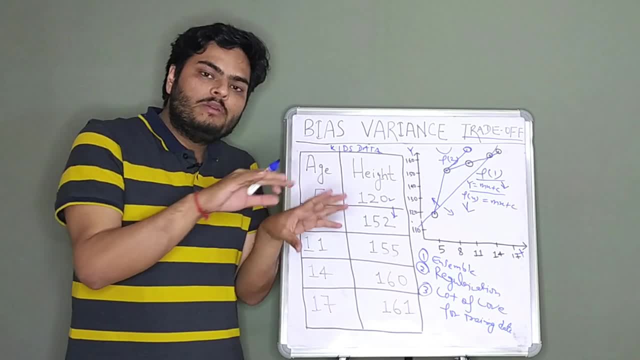 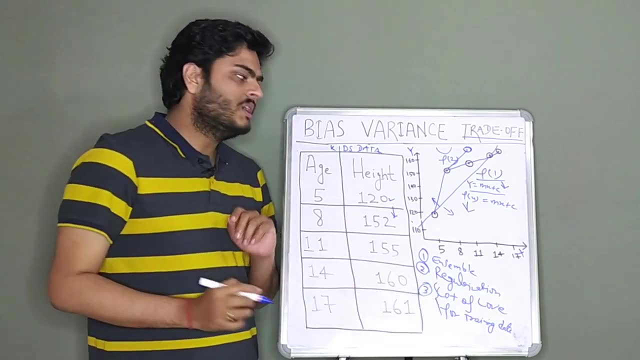 will try to actually break your data in many, many branches such that it can predict everything correctly, right? that is too much love for the training data. this is too much love for the training data, okay, and this is the model which is having a lot of love for the training data, okay. 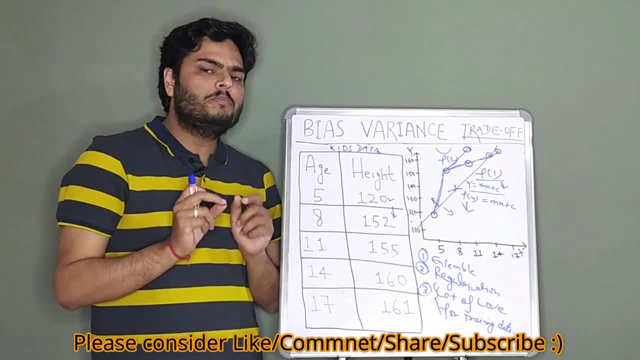 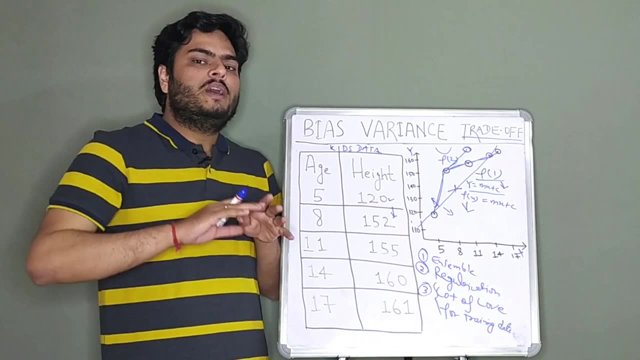 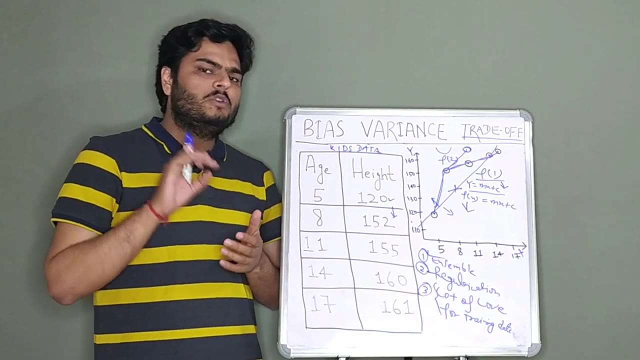 less love for the training data. this one thing you keep in mind, and then you will never forget the concept of high bias and high variance, and I told you to balance the bias variance trade-off. what we do is these things and sampling, regularization, these kind of things. okay, let me. 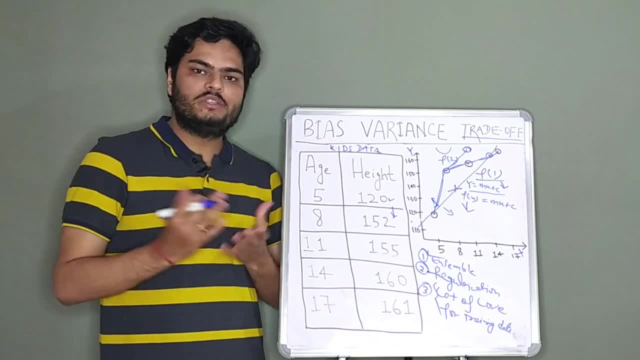 know what questions you have in mind. I'll see you all in the next video. till then, stay safe and take.